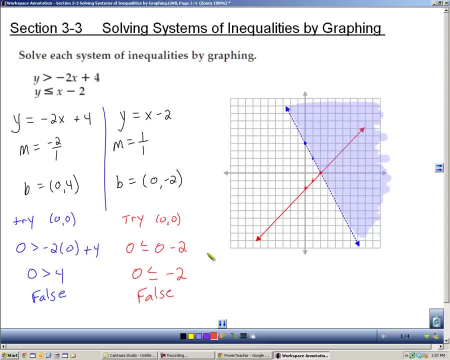 so I'm going to shade the bottom, because 0, 0 is on the false side. So now that we have them both shaded, we want to try to find any place where those two shaded areas overlap, And that would be right here in this region here. 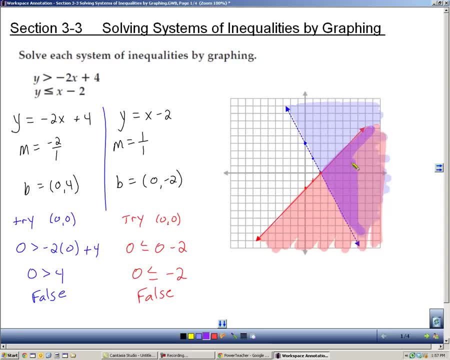 And so I make that a darker shade With your pencil. you just make sure that that's shaded in darker With the use of technology. here I'll just make it purple. So my solution is this: purple area. It's the only area that is overlapped. 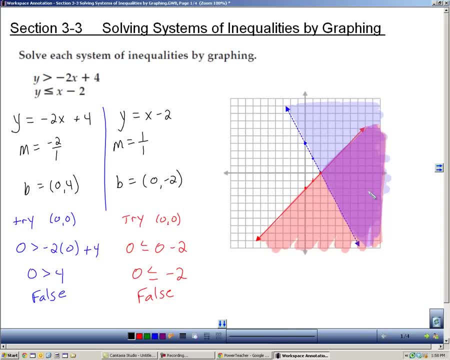 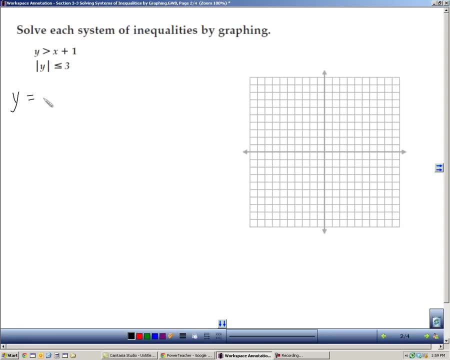 Or crossed by both the blue and the red area. So this dark area on the right is my solution. Here's our next example of inequalities. We'll start by graphing the boundary line of the first. So my slope is 1 over 1, and my y-intercept is at 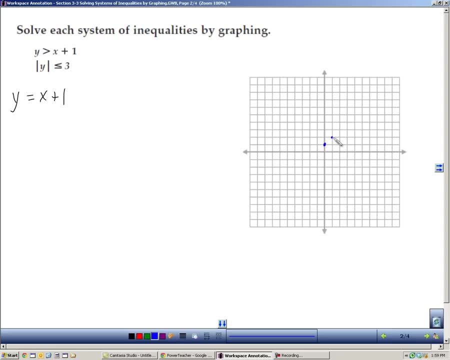 So here's: and 1, rise of 1, run of 1.. And because it's greater than I'm going to do a dotted boundary line, Let's go ahead and do the shading right away. I'm going to try a point. 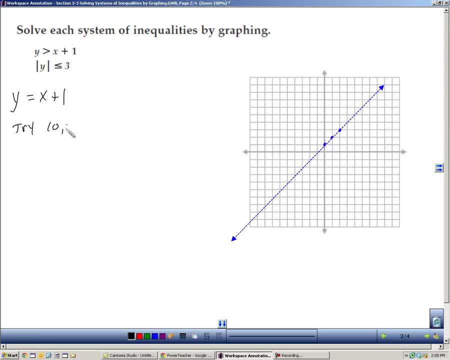 It looks like 0, 0 is on the right side, So I try that one. I plug in 0 greater than 0 plus 1, which 0 is greater than 1, that's false, So 0, 0 is on the bad side. 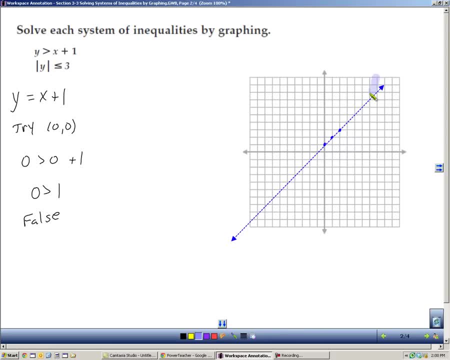 So I'm going to shade the upper left for this graph. So that's my first one. My second inequality is absolute value, which, if you remember back in previous sections we talked about, we can rewrite as positive: y is less than negative y. 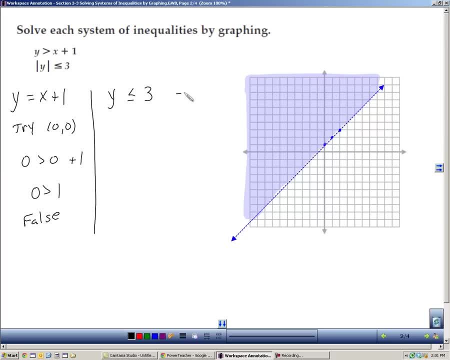 So that's my first one. My second, inequality, is absolute value which, if you remember back in previous sections we talked about, we can rewrite as positive: y is less than positive y. So that's my first one: Y is less than or equal to 3, or negative y is less than or equal to 3. 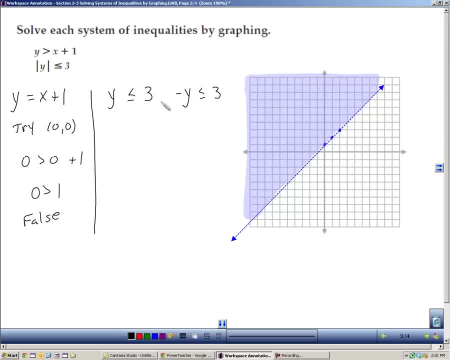 because the positive distance is smaller than 3, and so is the negative. So that actually creates two equations, two more lines. I'm going to graph This one: y equals 3.. And so we'll put that one up here. That is a horizontal line, and because it's less than or equal to, 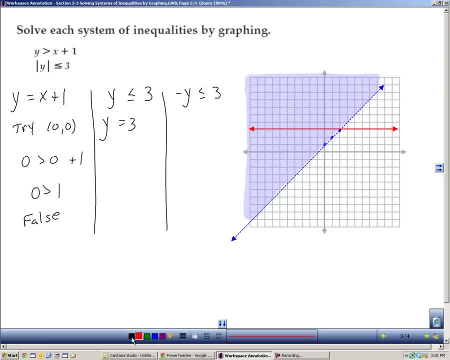 it's going to be a solid horizontal line. So there's the horizontal line. y equals 3, and now, if we plug in 0, 0, we get zero is less than or equal to three, which is true, which means zero. zero is on the true side. so I'm going to shade below this, below this line. 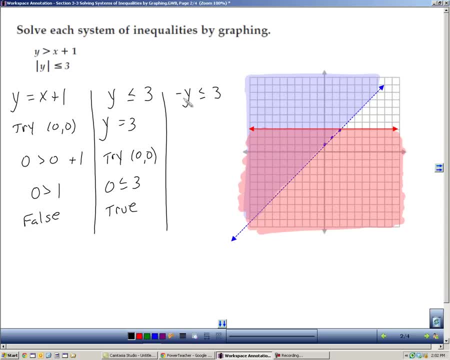 and then the last one I want to solve is here: negative y is less than or equal to three. whoops, the boundary line should be equal to, and then we divide everything by negative one, and so we make it: y equals negative three. so that line is a horizontal line down here at. 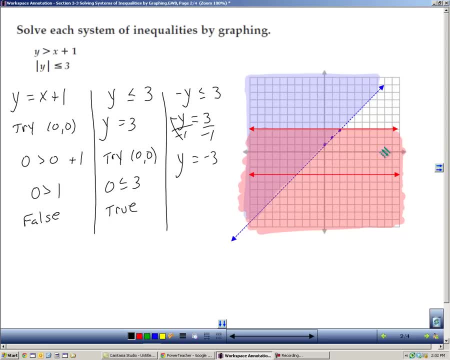 negative three. so there you see that line. I did it in red again and now we're going to try, zero, zero, to find where the shading is. so we say negative zero is less than or equal to three. well, that's true, because there's no such thing as negative zero. so zero, zero is on the good side. 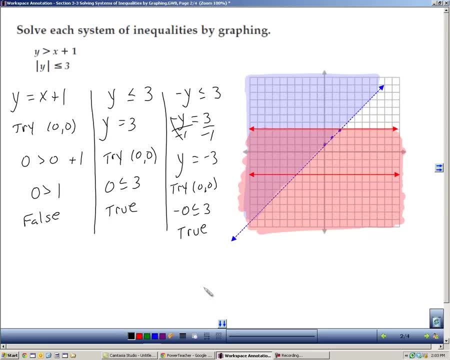 which means I want to shade up from that red line. so the point is my, my shaded region that has all three of them. you is below this upper red line- y equals 3, and then above the y equals negative 3, and it's to the left of the blue dotted line. 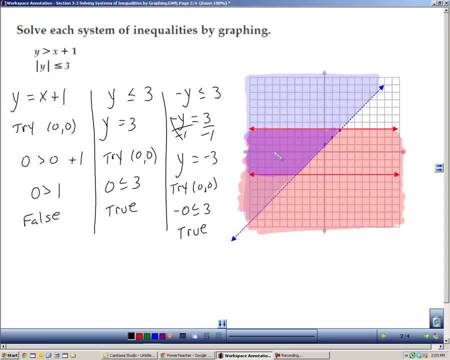 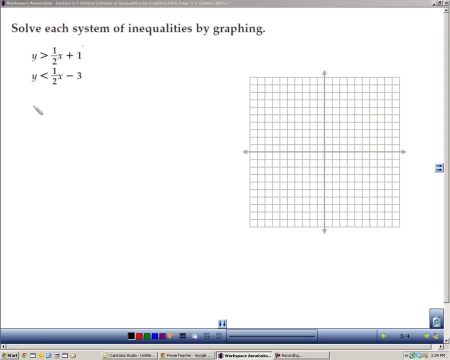 So that purple area that's in here, that is, all the ordered pairs in that region, will satisfy both of those inequalities. For our next example, I would suggest you pause it, try it for yourself and then come back and see what the answer is. 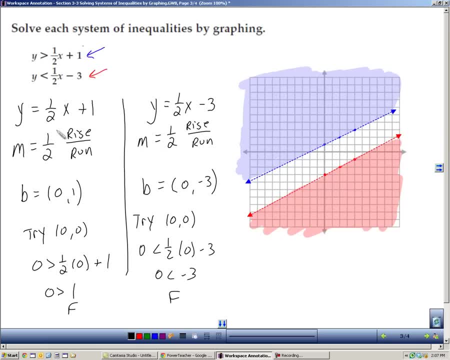 So here's the work with the first boundary line or the first equation: Slope is 1 half and the y-intercept is 0, 1.. So I do 0, 1 and go up 1 to the right 2, up 1 to the right 2.. 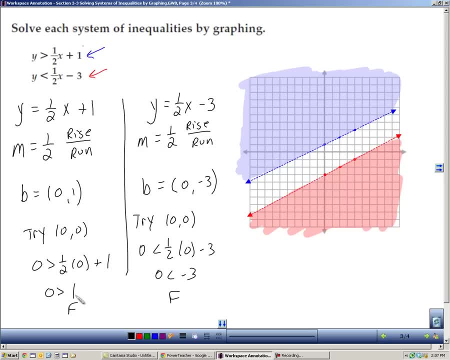 It's a dotted line because it's greater than, and when I plug in 0, 0, I get a false statement, which means I'm going to shade on the other side, the true side. Second boundary line is for the red one. 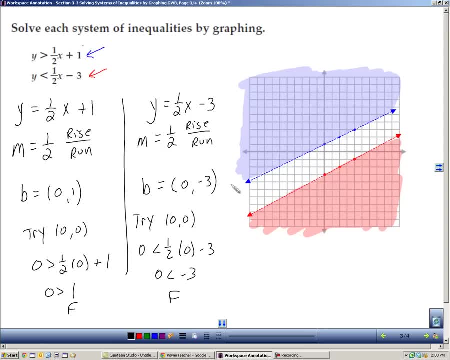 Again. slope is 1 over 2, rise over run. y-intercept is 0, negative 3, so I started down here, did up 1 to the right, 2 each time, did a dotted line again because it's less than.